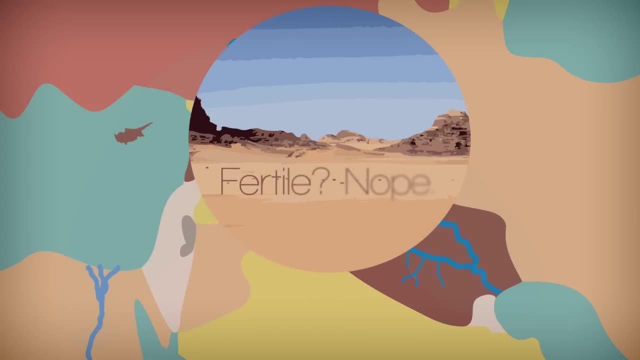 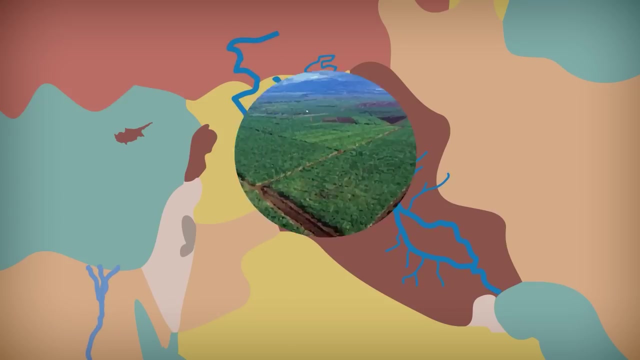 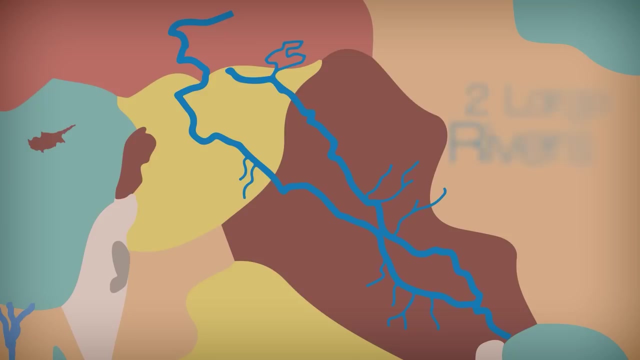 Crescent, not croissant. Most of the area isn't fertile at all. It's a dry, parched desert, But the great rivers that flow in the area were used to bring water to the dry land for farming. Today we are learning about two large rivers in this area that made civilization possible. 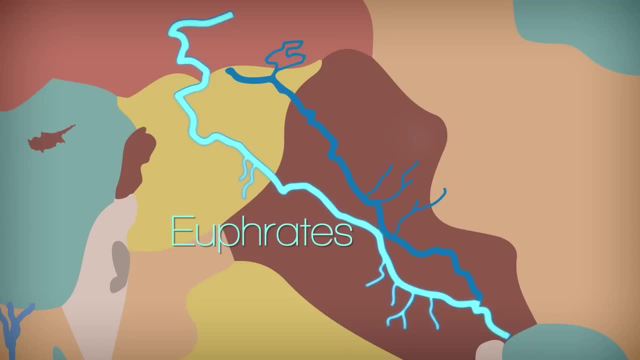 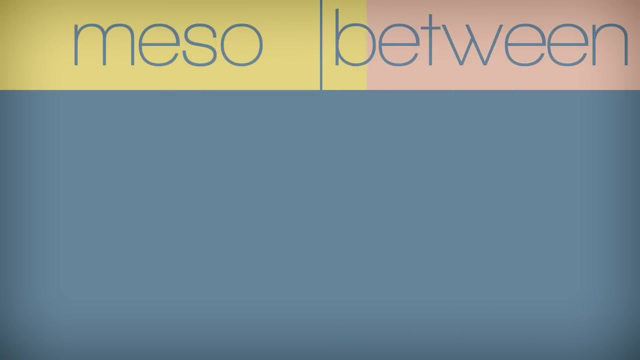 These rivers are called the Tigris and the Euphrates rivers. They stretch from modern-day Turkey down through Iraq and into the Persian Gulf. This area between the rivers was called Mesopotamia. Meso means between and Potami means river. 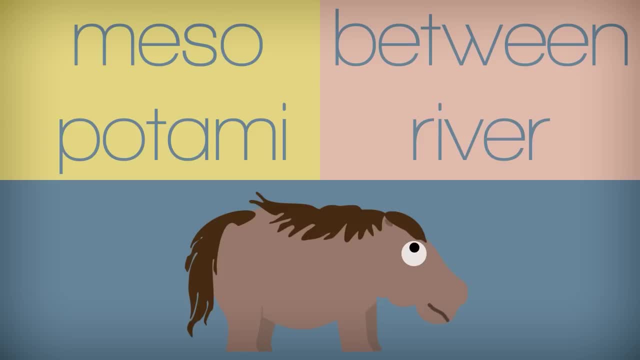 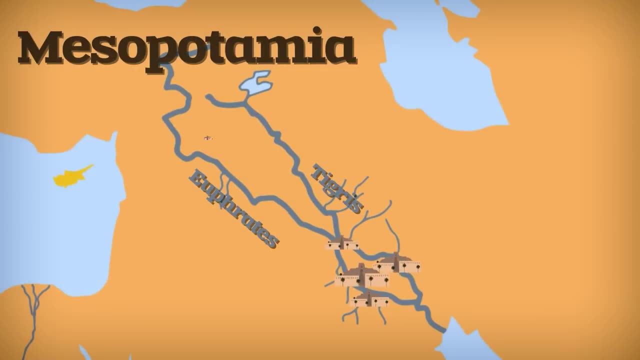 Kind of like how hippo means horse and Potamus means horse. Potamus means river, A river horse Kind of Many cities were built in Mesopotamia, including many with complex names like Kish, Uruk, Ur and Wasikani. 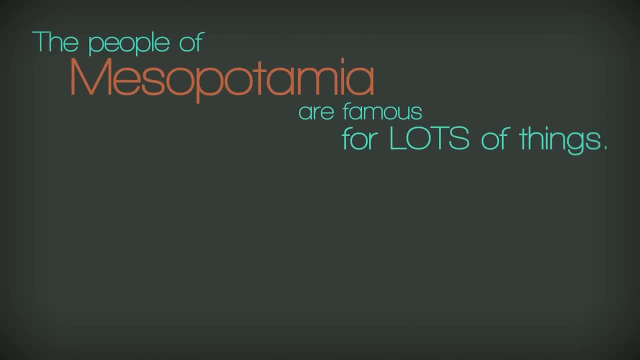 The people of Mesopotamia are famous for lots of things, including creating a system of riding, using irrigation to bring water from rivers to their farms, building huge cities out of mud, using some of the first wheels to spin pottery and later creating chariots. 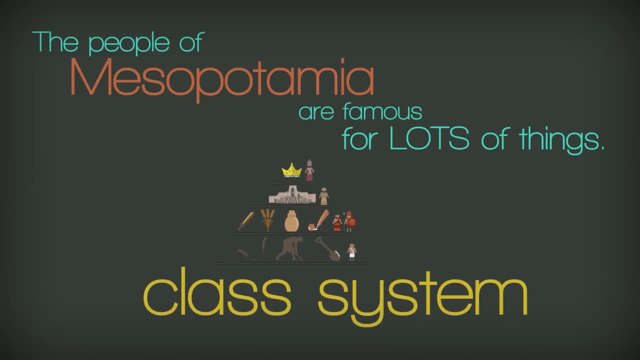 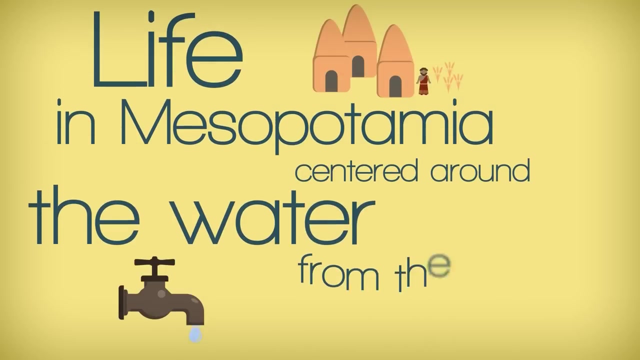 creating a class system of society, specializing labor and creating a system of laws and rules for their society. Most of these things were completely new to the world. at this time, Life in Mesopotamia centered around the water from the rivers. The rivers in Mesopotamia can be unpredictable. 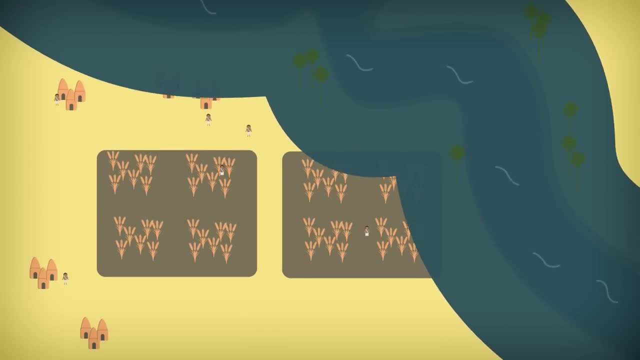 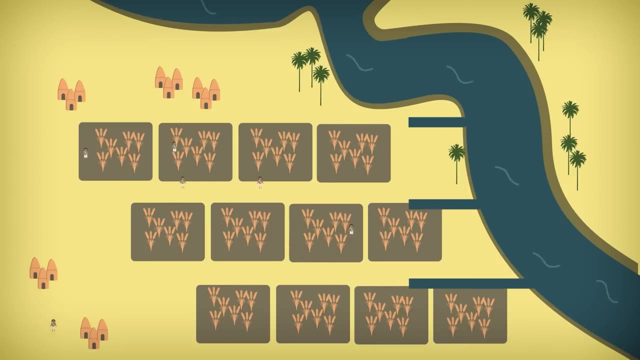 Sometimes a big rainstorm comes and runs through the river. Sometimes a big rainstorm miles away can make the river fill up too fast and flood their homes and farms. The farmers had to dig canals to bring the water to their farms and also build dams. 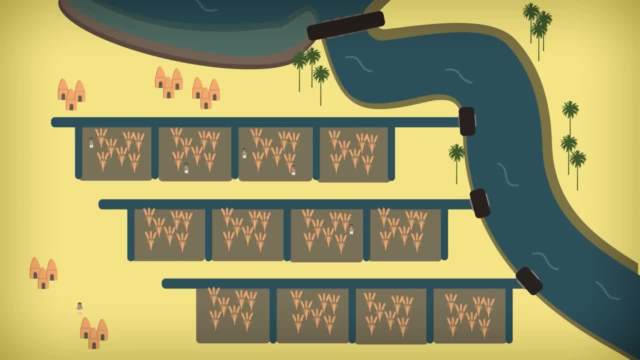 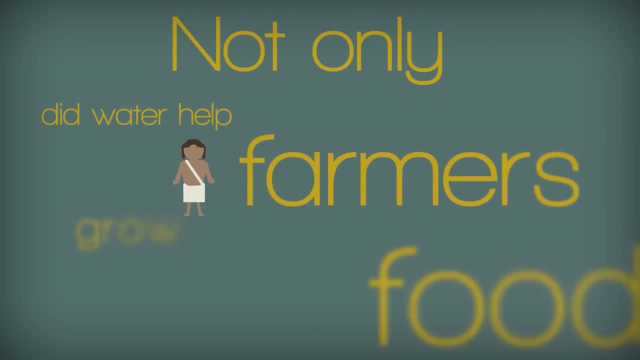 levees and gates to keep the rivers from flooding their homes and farms. A bad flood could wash away their crops, so they had to protect them. Not only did water help farmers grow food, but it also helped skilled workers make mud. Yes, 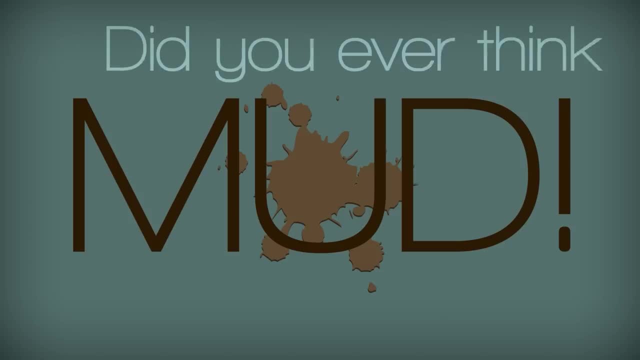 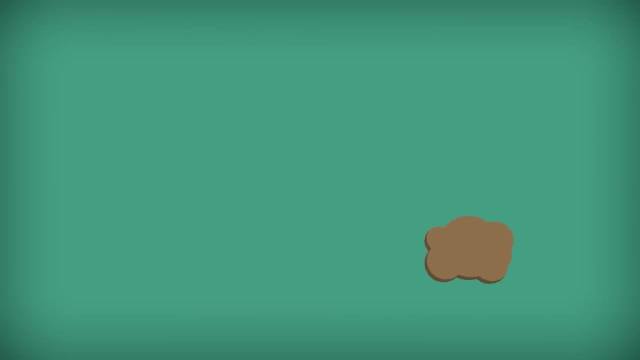 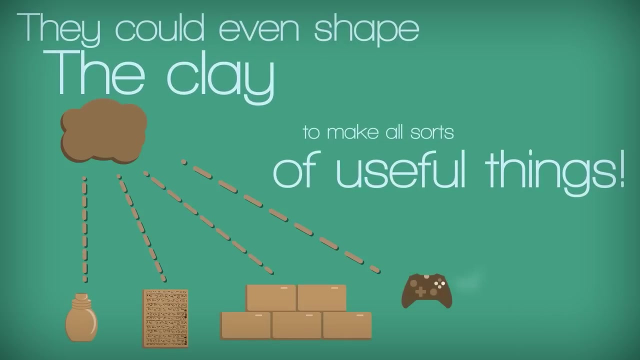 Mud, Wonderful, Amazing Mud. Did you ever think mud would be such a big deal In Mesopotamia? the mud was thick like clay And when it dried it was hard. They could even shape the clay to make all sorts of useful things. 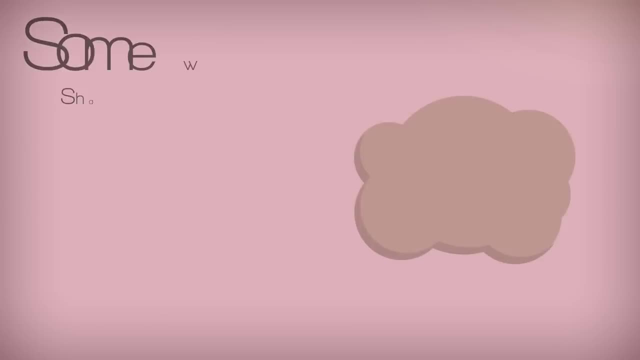 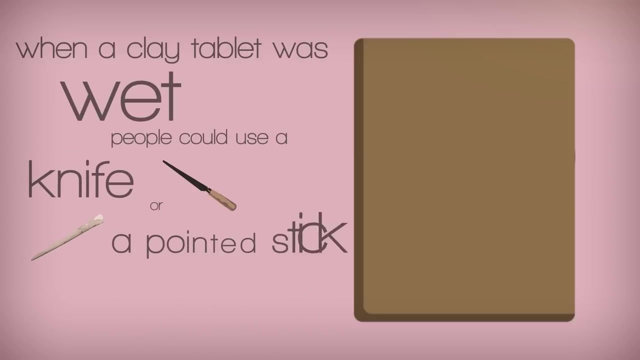 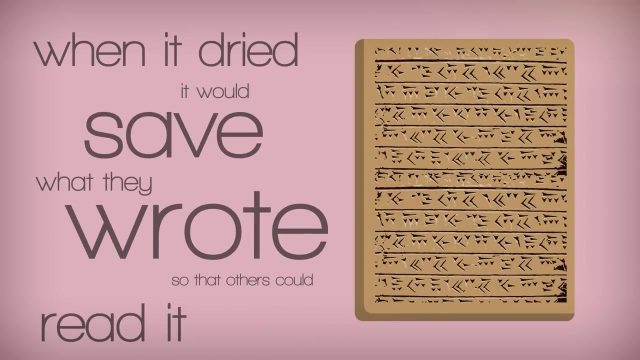 Maybe not that Some workers shaped clay into tablets. When a clay tablet was wet, people could use a knife or a pointed stick to carve simple symbols and writing into the clay tablet. When it dried it would save what they wrote so that others could read it. 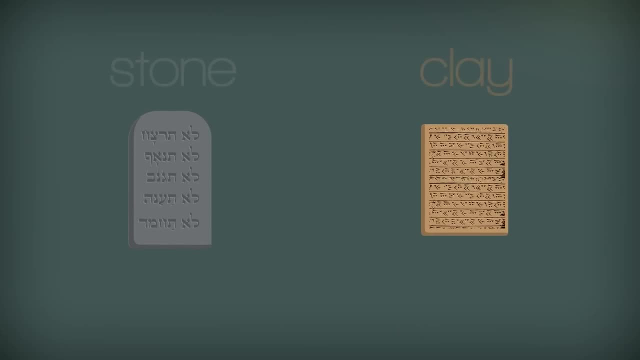 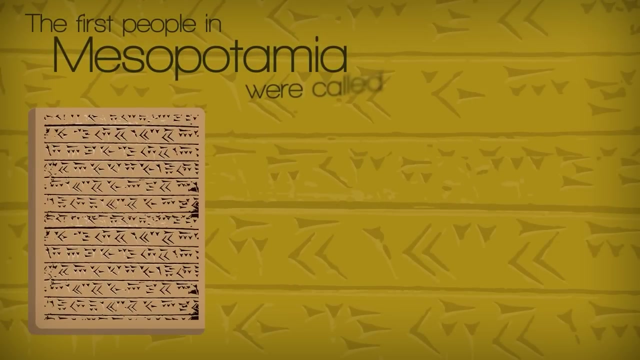 This was so much easier than chiseling into a stone tablet and much lighter to carry around. Plus, there's just a lot of clay in Mesopotamia. The first people in Mesopotamia were called Sumerians. They had their own system of writing that today we call cuneiform. 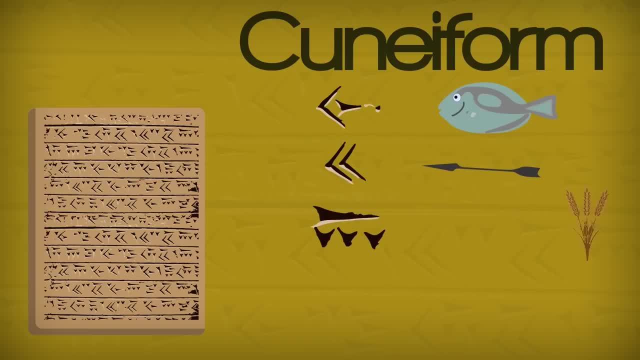 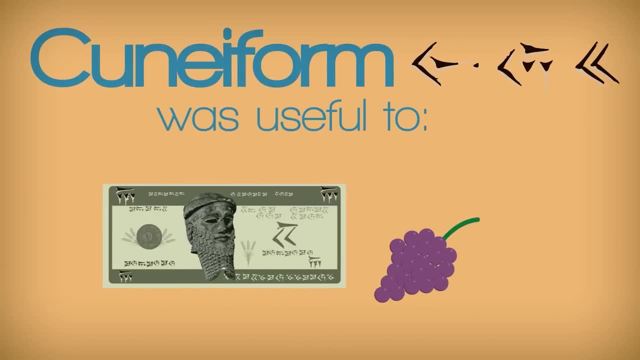 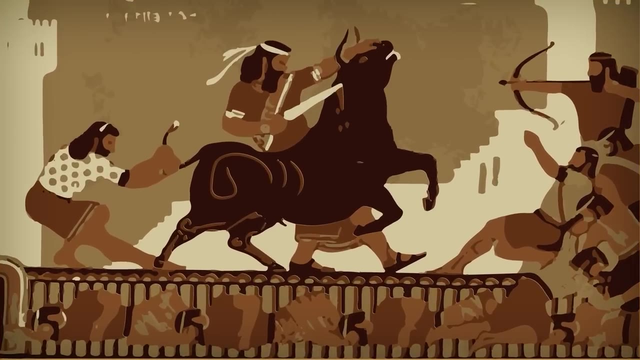 Cuneiform uses little wedge-shaped impressions and lines to represent words and ideas. Cuneiform was useful to keep trade records, write rules and laws, keep a history and even write stories and poems. One of the oldest writings we have preserved is a poem called the Epic of Gilgamesh about 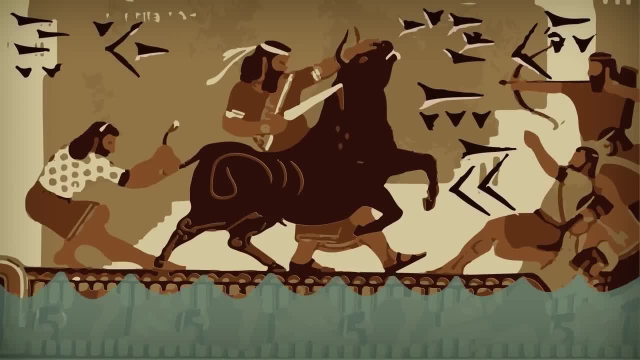 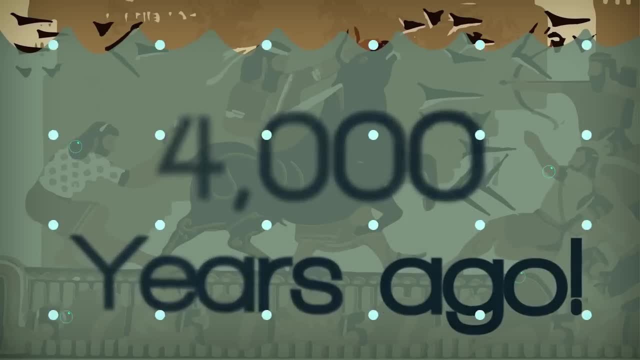 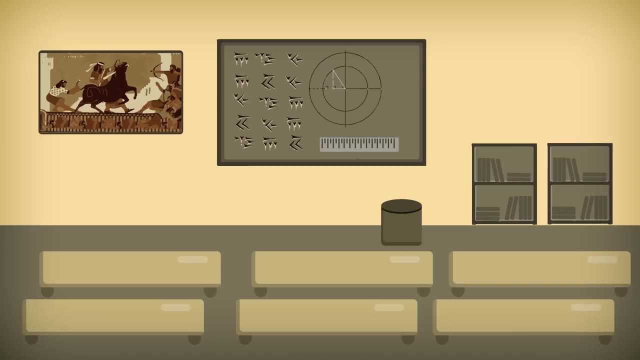 a king from Ulric and his adventures. It also features a story about a great flood that covered the earth. The story was written about 4,000 years ago. The Sumerians started schools to teach people cuneiform and other things like math. 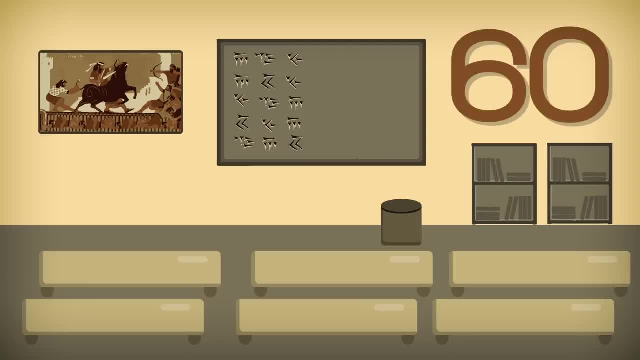 They used a number system based on the number 60. They used the number 360 to measure degrees and angles to create a perfect circle. They measured time using 60 seconds for 1 minute and 60 minutes for 1 hour. They even invented the sundial, the first known tool that measured time. 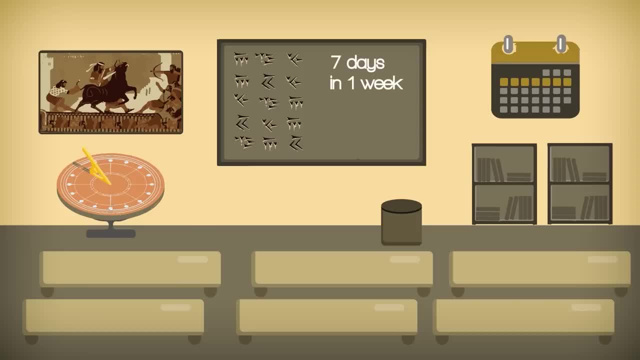 They also created a calendar with 7 days in a week and 12 minutes in a week. They also created a calendar with 7 days in a week and 12 minutes in a week. They also created a calendar with 7 days in a week and 12 minutes in a week. 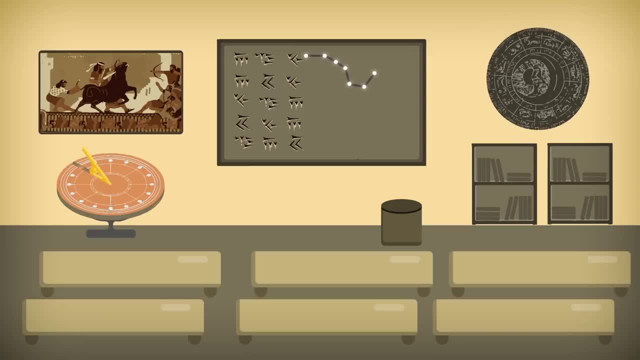 It was about 12 months in a year. based on the stars, constellations and planets they observed in the sky, This was the beginning of astronomy, or the study of space. We are still using a lot of this today. Another great use for clay in Mesopotamia was bricks. 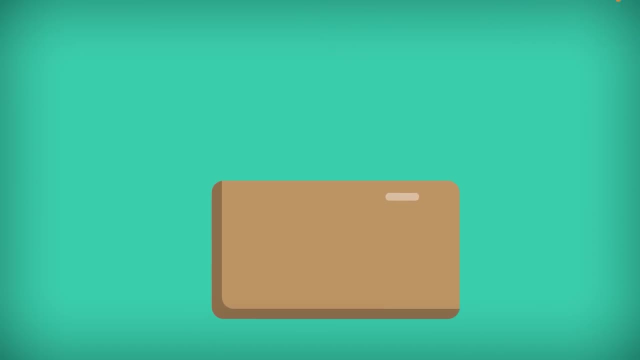 The bricks could be hardened by drying in the sun or made really hard by baking them in a fire. The people of Mesopotamia built large cities out of these bricks. One of the most amazing types of buildings that they built with clay bricks were Cretaceous. 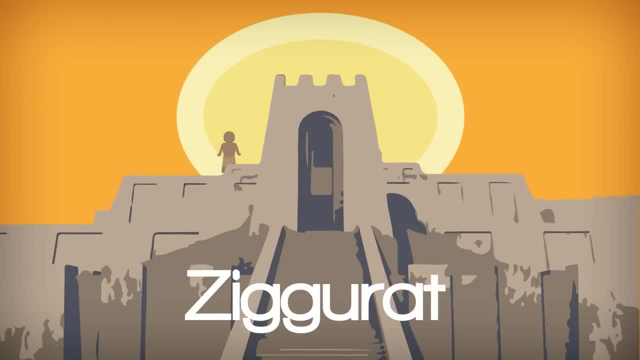 They were also built using bronze putches, called ziggurats. Ziggurats were tall structures or temples with steps up them all the way to the top. Only the priests, priestesses and other religious leaders could go to the top. The people that built the ziggurats worshipped many gods. 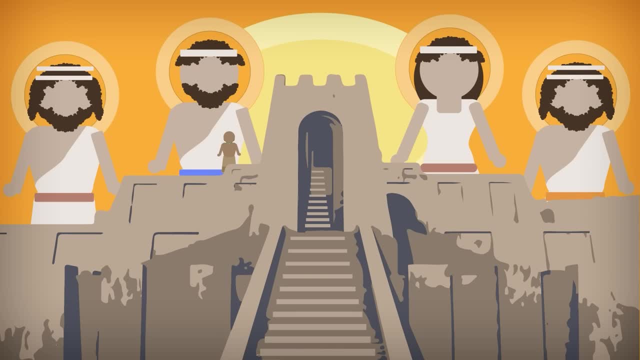 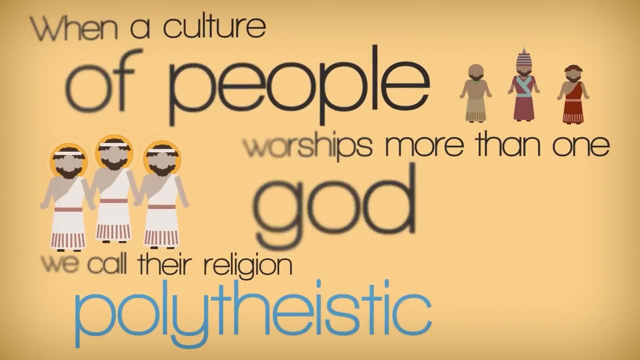 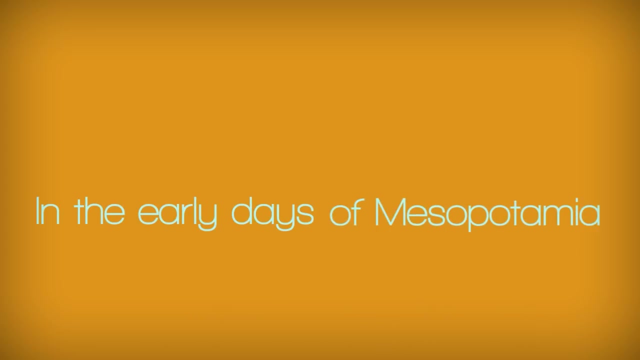 In fact, each city had its own special god that they worshipped. mainly When a culture of people worships more than one god, we call their religion polytheistic. Poly means many and theism means belief in God In the early days of Mesopotamia. 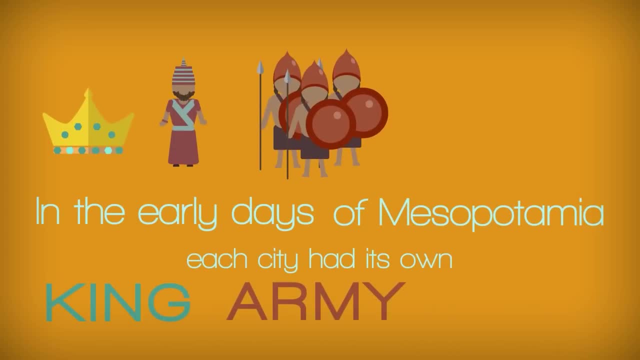 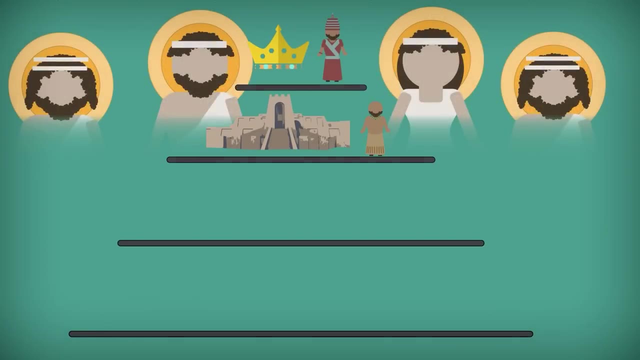 each city had its own king, its own army and its own rules. The king and the priests were the most important people in the cities. They would tell the people what to do to keep the gods happy. Merchants, traders and artisans were part. 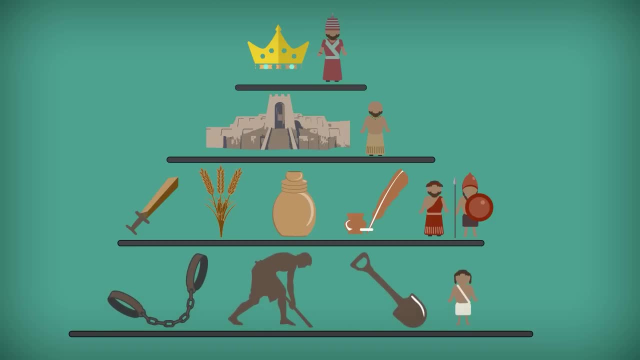 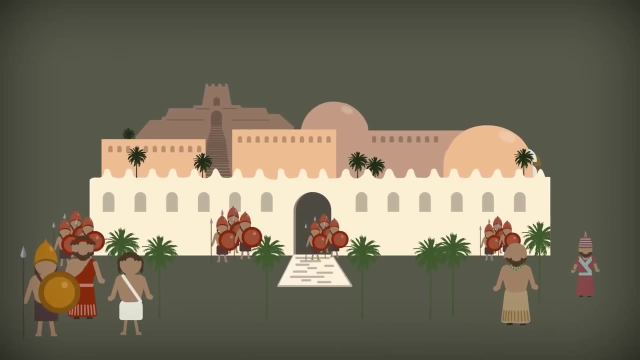 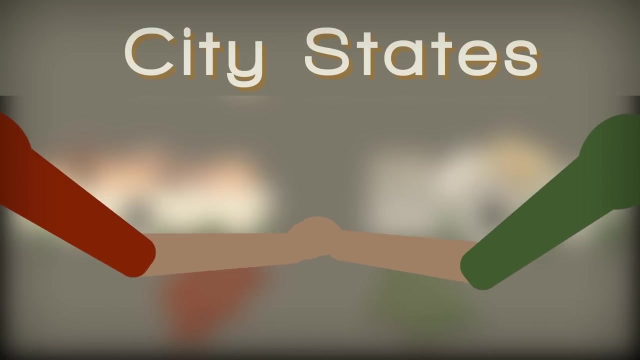 of the working class of people and slaves were at the bottom of the social structure. Everyone in the city paid taxes for the gods, to the priests and the king. The taxes were used to run the kingdom. These little kingdoms were called city-states. Sometimes the different city-states got along, Other times they didn't. 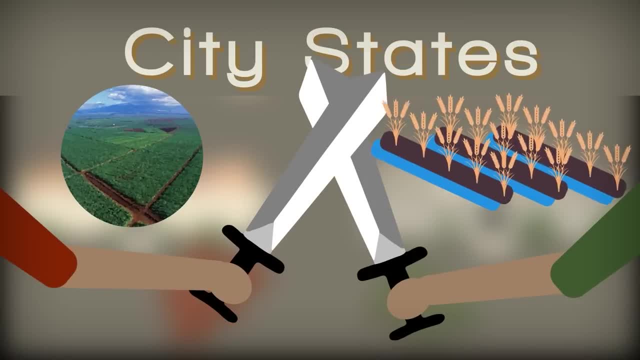 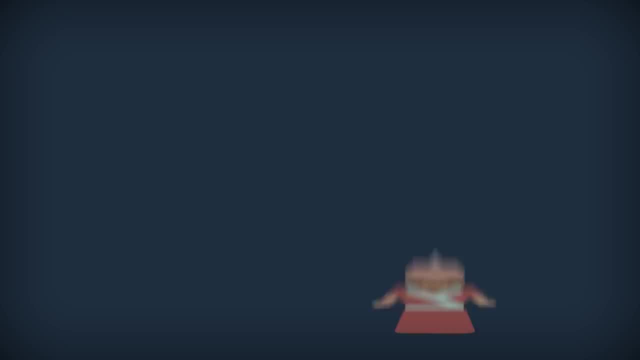 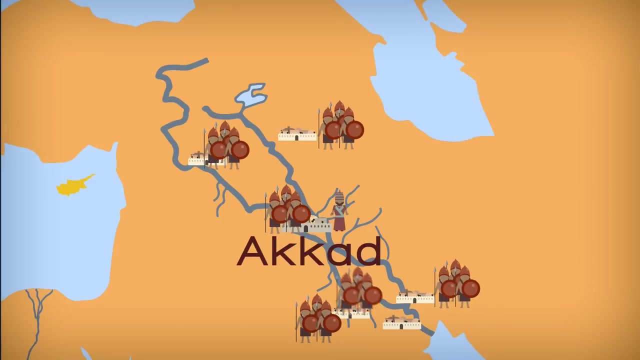 and they fought. They would fight over land, water and other things. Sometimes the losers in the fight would become slaves. One of the city-state kings was named Sargon. He was the king of Akkad. He used his army to conquer other city-states and create a unified empire. 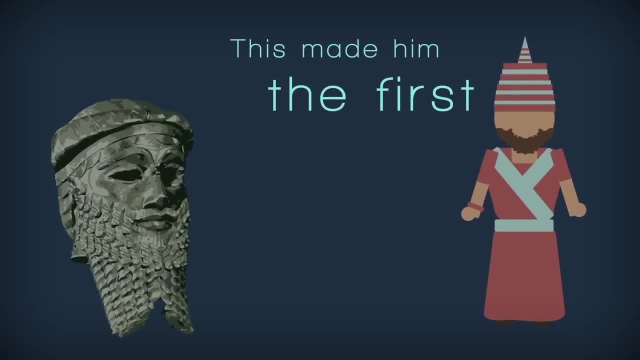 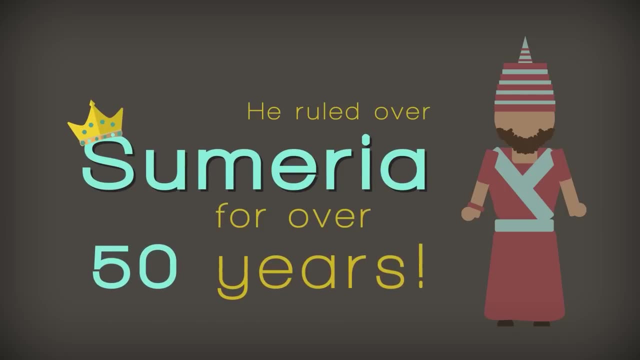 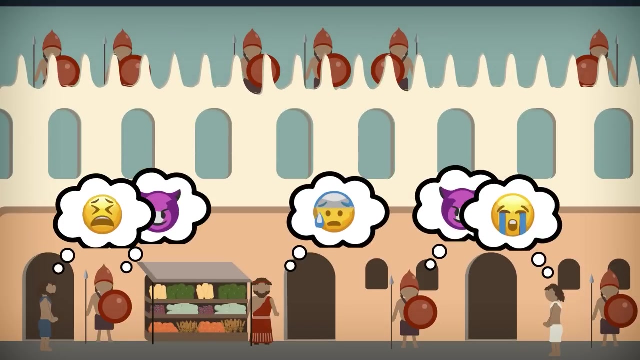 called the Akkadian Empire. This made him the first great king in history that we know of. He ruled over Sumerians for over 50 years. He used his army to keep other cities afraid The people would obey, even if they weren't happy with him as their ruler, because they 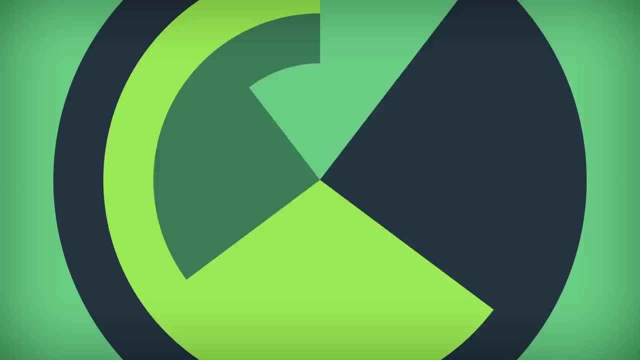 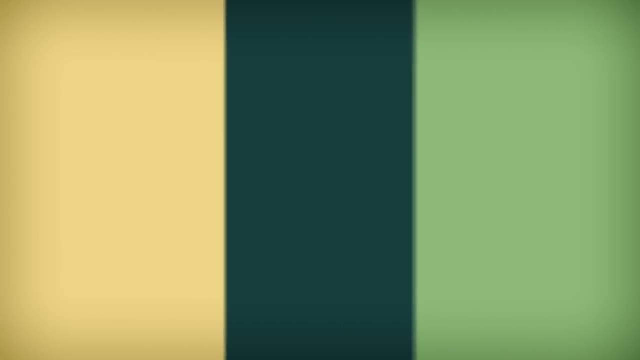 were scared. Sounds fun, right. Eventually, Sargon's empire fell. It fell to his northern rival, Babylonia, which is a story for another video. Even though their empire didn't last forever, many of the inventions and achievements of their civilization 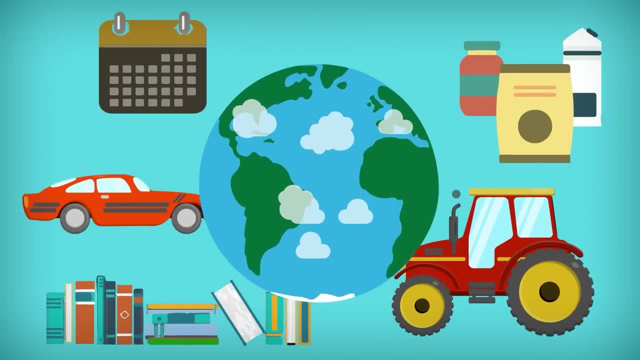 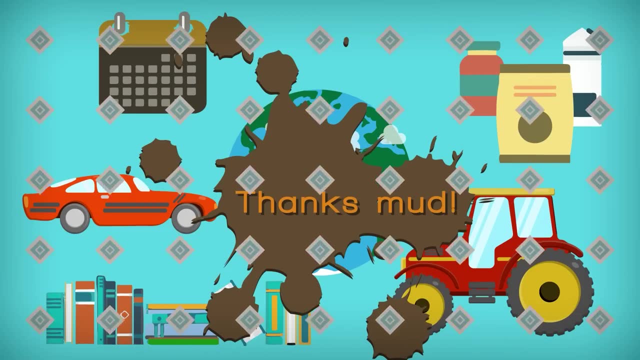 impact our lives today. So look around our modern world and notice just how many amazing things we have. And they all started with a group of people playing with mud. Thanks, mud. If you like learning about history, check out our other videos And don't forget to.